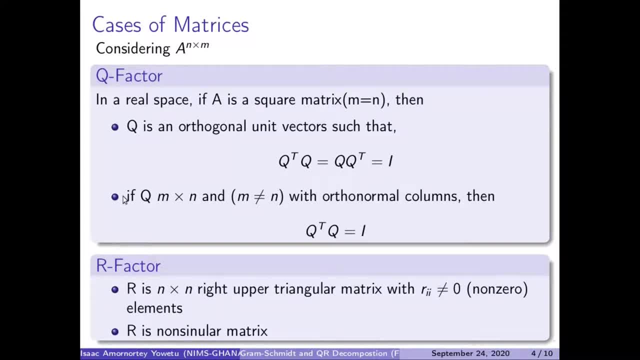 matrix here. In the case where our Q of size n by m and our m is not equal to n with autonomous columns, then we have our Q transpose times Q, which gives us an identity matrix, And considering our R factor, Our R figure will be equal to Q transpose times MOur. R factor will give us an identity matrix here. 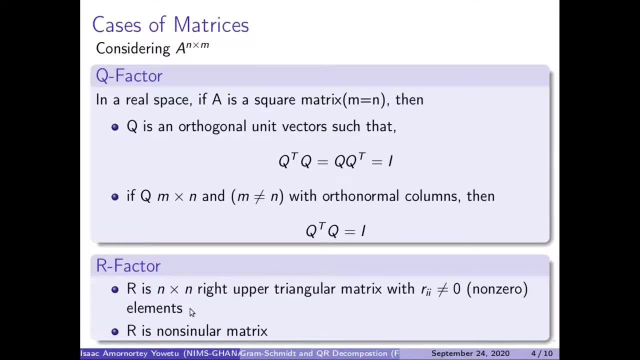 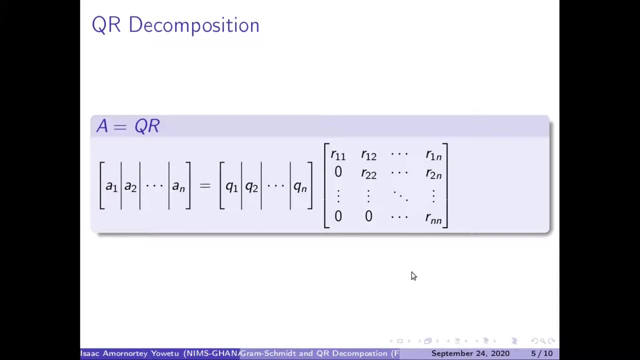 And considering our R factor, our R factor will be equal to Q transpose times Q, which will factor will always be n by n. right upper triangular matrix with the diagonals being non-zero elements and our R is always non-singular matrices, and this is our QR. 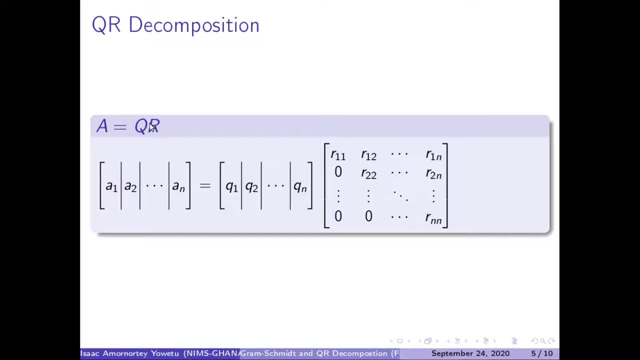 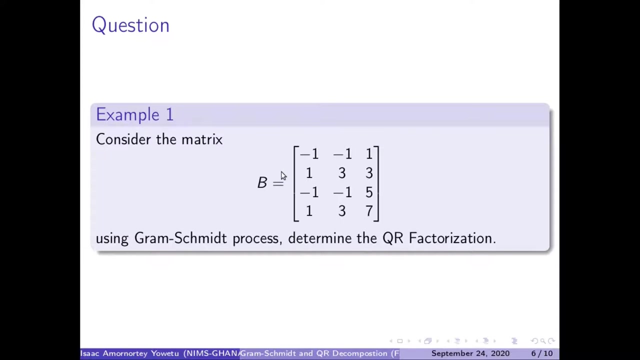 decomposition. when you have a matrix A, you can decompose it with the following columns, that's A1 to AN. we can decompose it towards the following columns like: Q1 to Qn, and in this our right upper triangular matrices are here. so we want to understand how will be able to do the QR decomposition from. 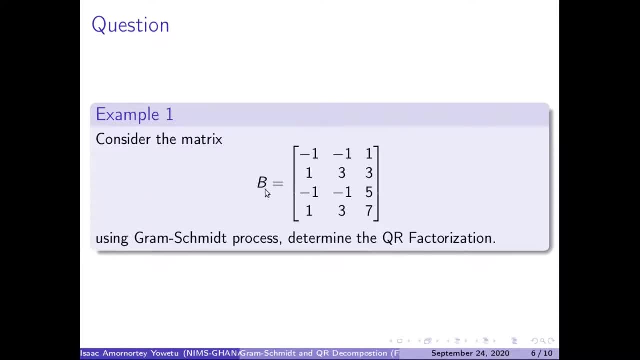 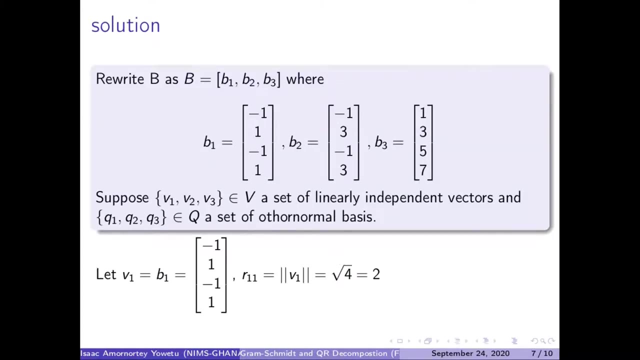 this example as considering the matrix B, which is the whole of these, that's 4 by 3. using the Kleinsmeier process, determine the To solve that we rewrite our b into the following columns, that is, b1,, b2,, b3, where there is. 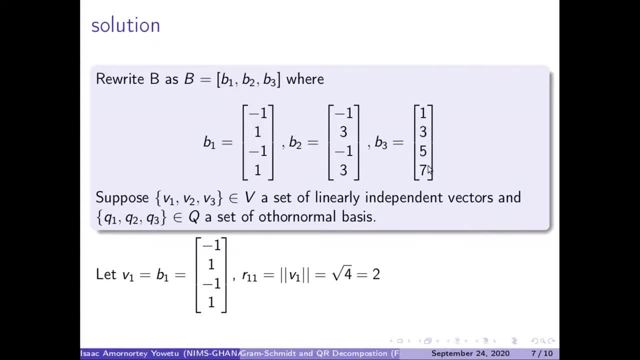 our b1 vector, b2 vector and our b3 vector. So we now suppose another vector that is going to help to aid in the computation. We have v1, v2, v3 belonging to the b-space, of which there are a set of non-linear independent. 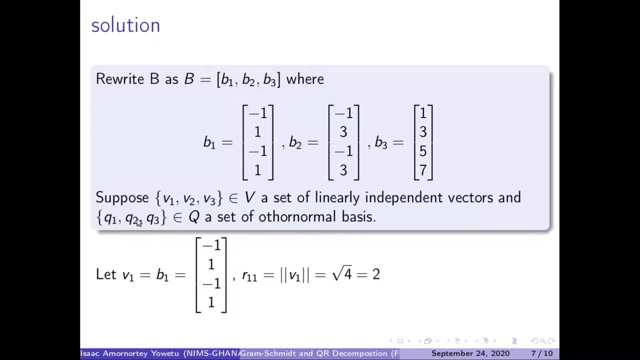 vectors and our q1, which we are interested in- q1,, q2,, q3- belonging to the q matrix, also a set of autonomous bases. So we then go ahead to solve the problem that has been given. So, first of all, we let our v1 to be equal to b, which is the same as the matrix that. 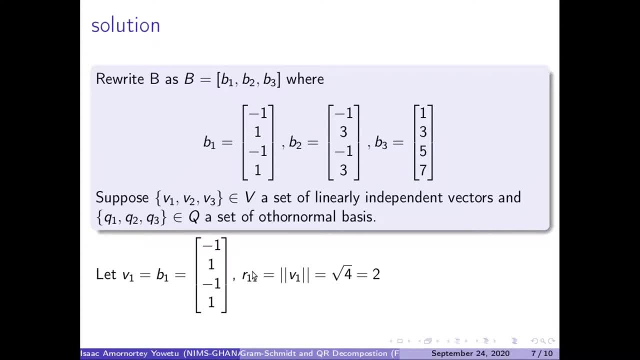 we have here. We calculate our R11 index. Here is the length of our v1, and that's the very truth that we have here. We will find the length of it or the number of it we will get to. That's what we have here. 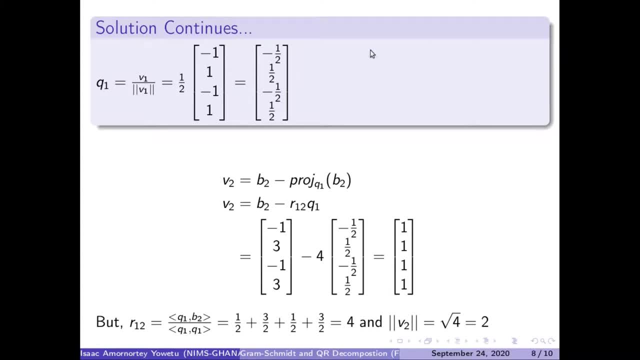 Okay, now, having obtained our q1 here, our v1 here, we know the length of or the number of v1 is equal to 2.. So 1 on 2 times our v1 vector here happens to give us 1.. 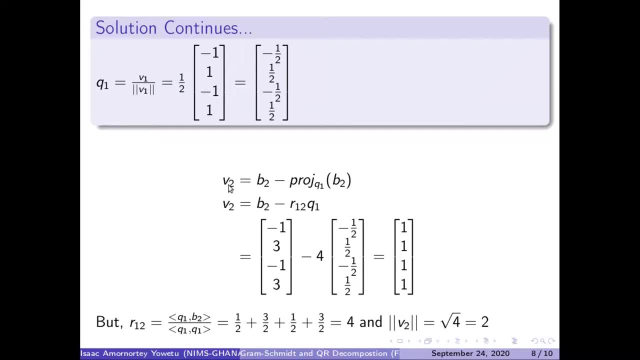 We then go ahead to find our v2, which it can be expressed as b2 minus the projection of b2 onto q1.. We can rewrite our v2 as b2 minus a certain scalar from our row 1, column. element of row. 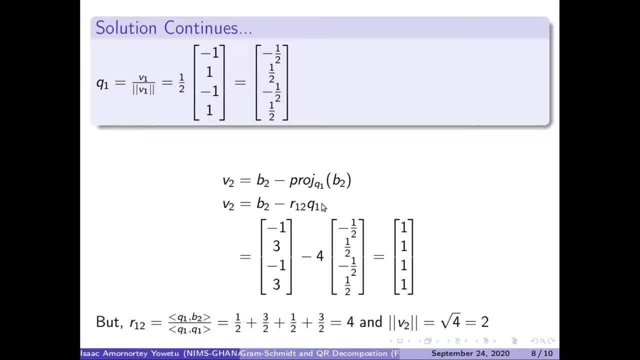 1 column, 2 times our q1 vector. Okay, So that's it, Thank you. We will then do the same thing with our q1 vector here We will have, of which we have our b2 vector to be here, this one, and we find the inner. 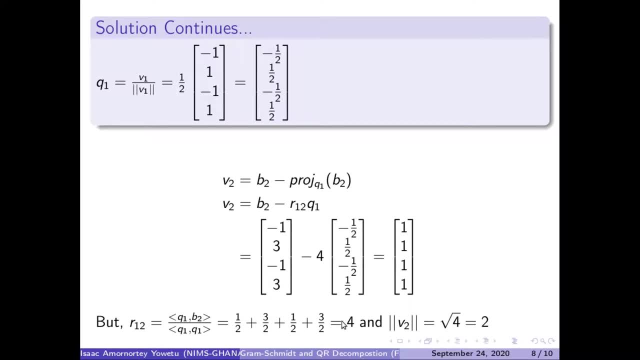 product of the whole of this one, we will get 4.. So 4 times our q1 vector here. when we do that simplification, we will be getting 1, 1, 1, 1. here Now, having obtained our v2, we find the length of it or the number of it, which gives us 2.. 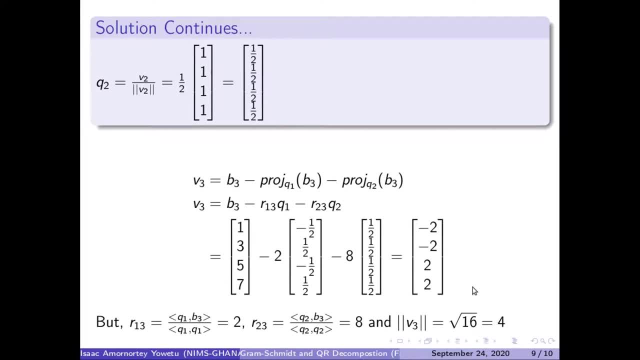 Okay, Okay. And also being able to obtain our V2 vector here, we find we already know the length of it, so we just multiply 1 over our 2 here, which 2 is from the norm of 2 times our V2 vector. 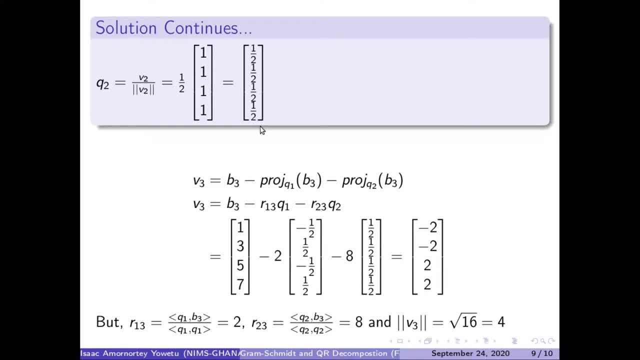 here happens to give us our Q vector here. Okay, now we continue. So to get our V3, we have pins to have our V3, minus the projection of V3 onto Q1, minus the projection of V3 onto Q2, which we can rewrite this one as V3, as in the terms of: 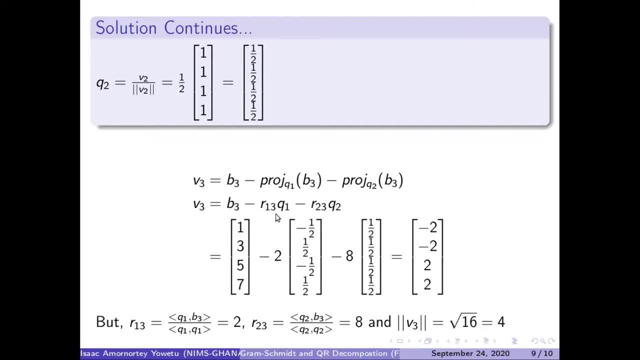 this expression: V3 minus a certain scalar, R13 times our Q1 minus R13.. Okay, Okay, Okay, The element of row 2, column 3, from our right upper triangular matrix times our Q2 vector, of which Q1 and Q2. we already obtained it from our previous calculations. 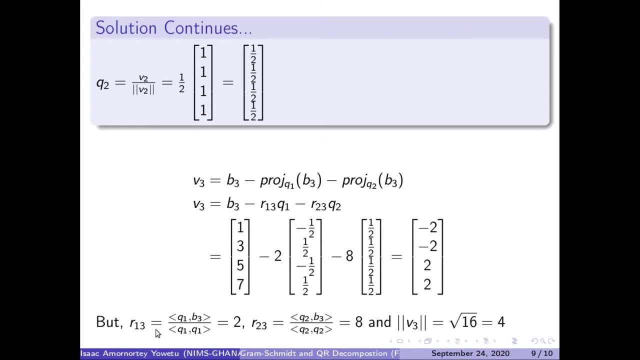 So to get our R, row 1, column 1, for the right upper triangular matrix, is the inner product of Q1- B3 on the inner product of Q1- Q2.. Q1- Q1, which the denominator will give us 1, so we cannot focus on the numerator which. 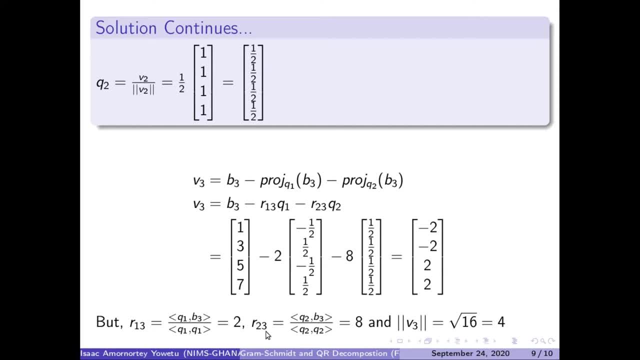 is 2. when we come to the second element, our R2, R2, row 2, column 3 element is the inner product of Q2, B3 on Q2, Q2, which the denominator as well will also give us 1, so the numerator. when you find the inner product of the numerator, 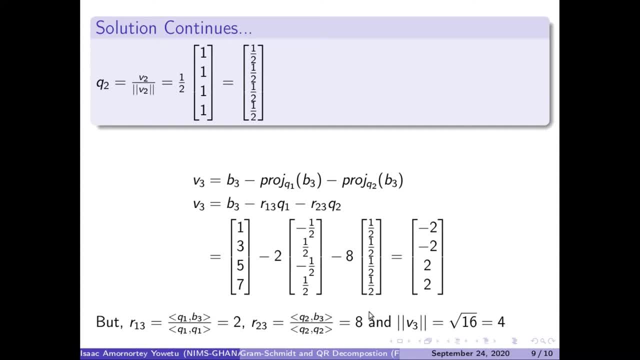 Okay, Okay, Okay, Okay, That's it also give us what 8? then we just substitute it back here, which we know our Q1, Q2 and V3. so substituting it here, we eventually get this vector. here, that's our V3 vector. 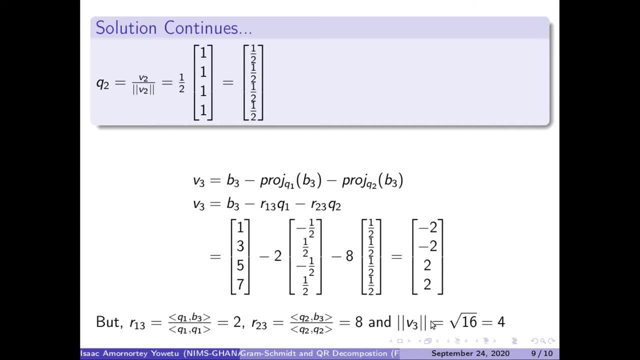 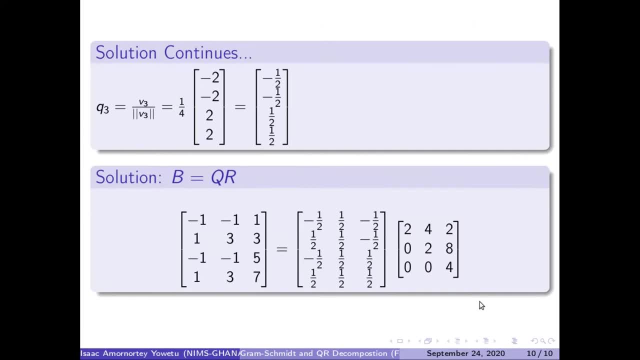 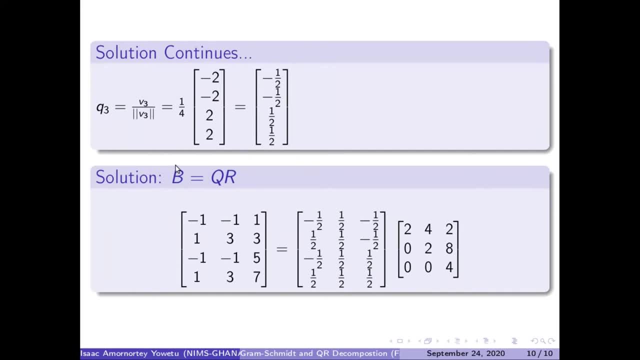 Q3 vector here. So in conclusion, we say our, our matrix big can be to decompose to Q and our r, which is a very solution that we happen to obtain here, our q, all well, an autonomous basis, or which, a very solution that we happen to obtain here, our